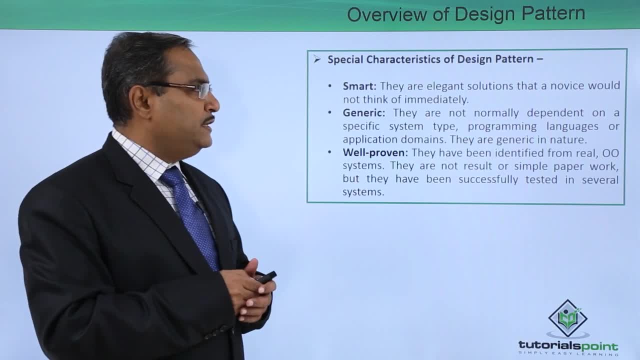 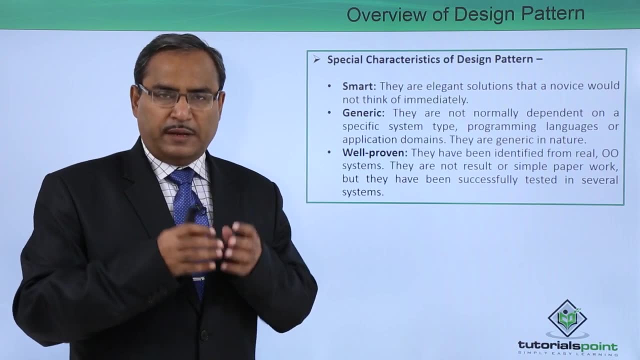 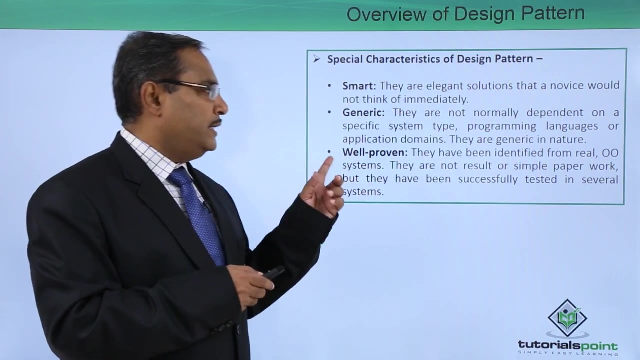 smart. They are elegant solutions that a novice would not think of immediately. So this is a smarter solution. So one novice software developer, he or she may not get this idea at the beginning. Generic, They are not normally dependent on a specific system, type, programming languages or application. 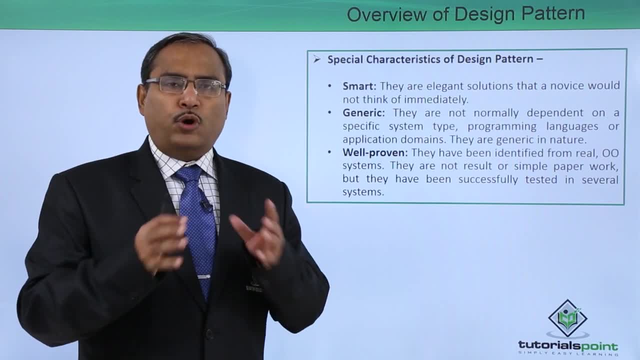 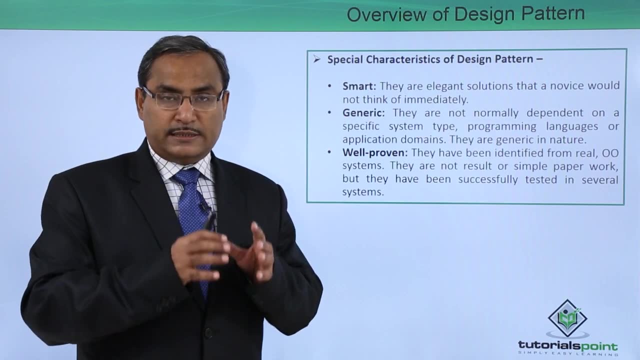 domains. They are generic in nature. Obviously, the programming language should be object oriented. So it is not like that the design pattern is only applicable for NET. Design pattern is only applicable for Kotlin or, say, Java. It is not like that. It is generic in. 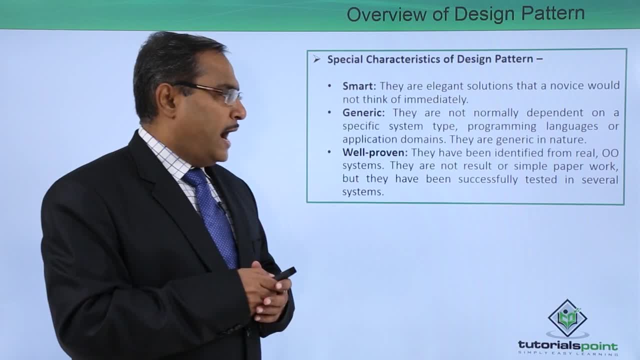 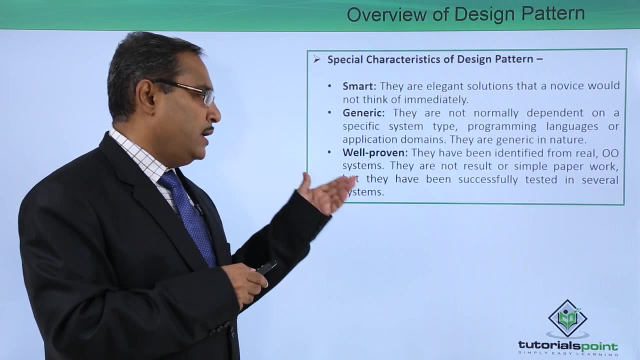 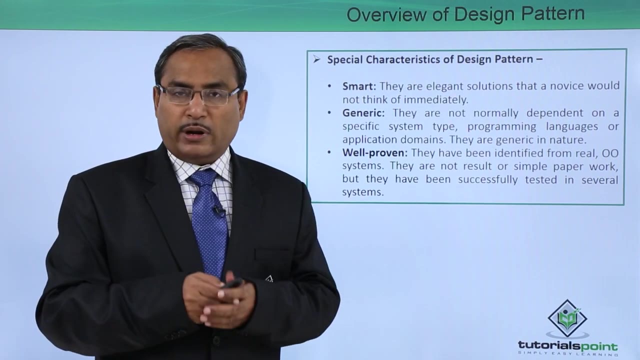 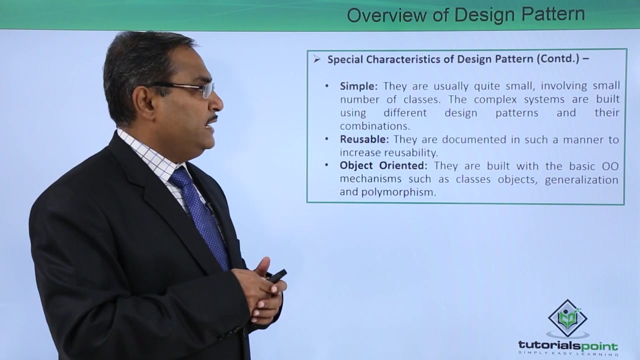 nature, Well proven. They have been identified from real object oriented systems. They are not result or simple paperwork, but they have been successfully tested in several systems and several systems. after getting implemented, they are working fine, So simple. Next property, next characteristic property of design pattern is simple. They. 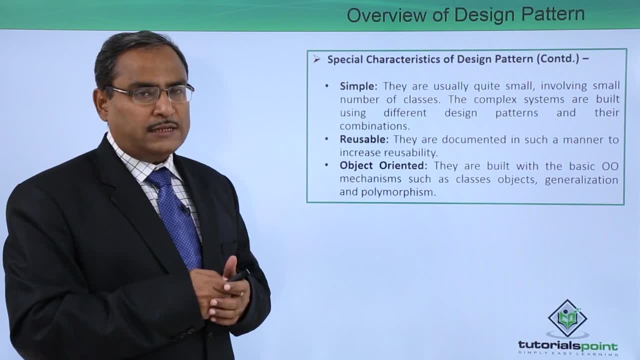 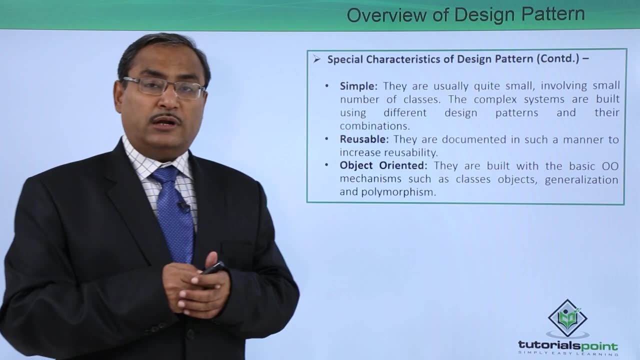 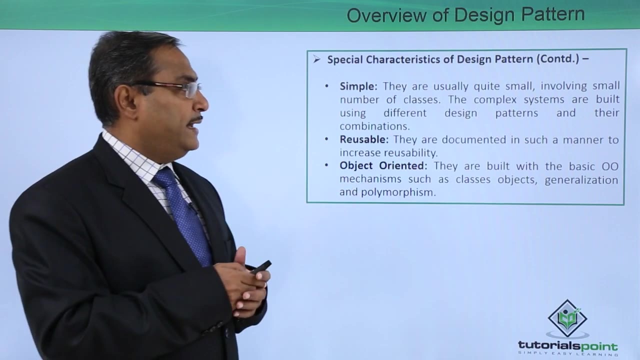 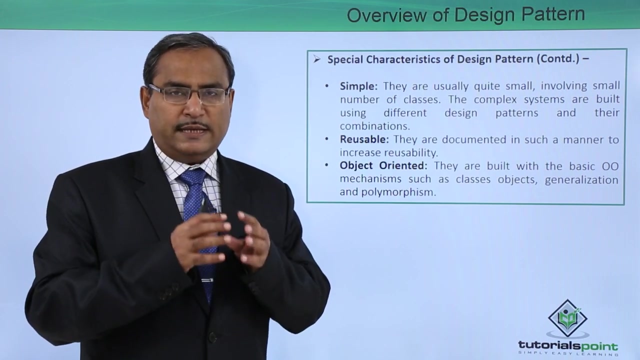 are usually quite small, involving small number of classes. The complex systems are built of different design patterns and their combinations. It is not like that only one software will have only one design pattern. There may be collection of multiple design patterns in the implementation and always design pattern tries to make the optimum number of classes. 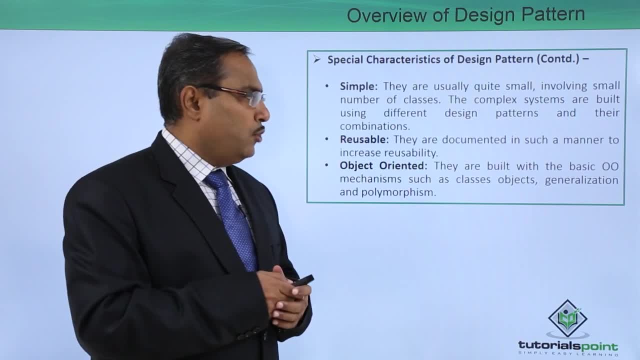 are getting used, Reusable. They are documented in such a manner to increase the reusability. We programmers, we developers, always believe on this particular thought. that is a reusability. But the reason that we are Usable is because we are a software that is used for design. So, for example, a 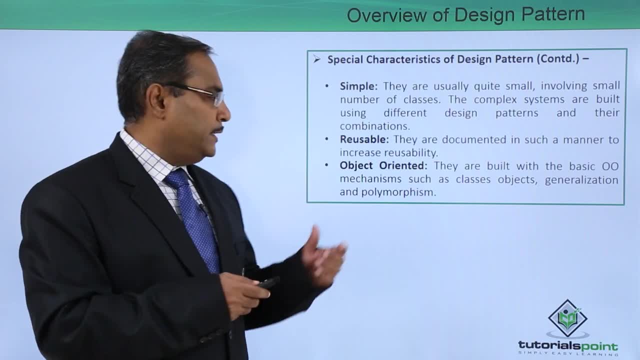 software that is used for design. In that case, a software that is used for design is used for design. We are using software exactly the same as design is used for design. We are using is a reusability: Object oriented. they are built with the basic object oriented mechanisms, such as classes. 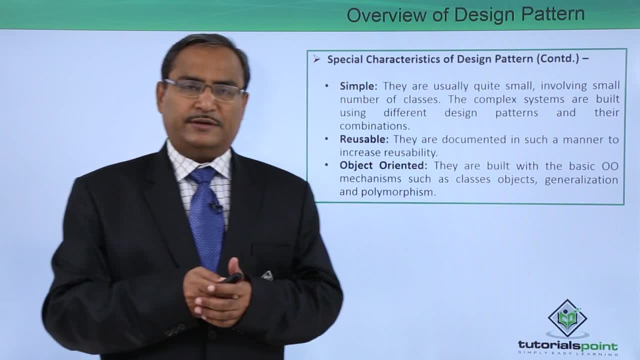 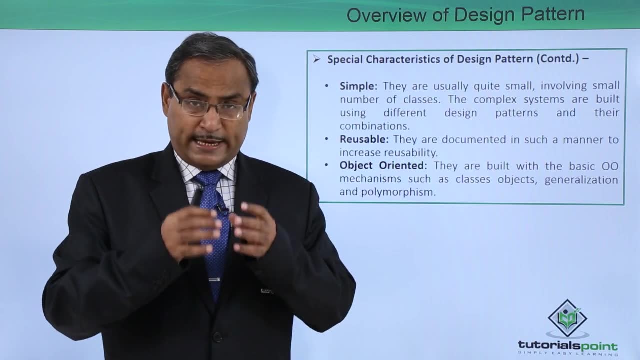 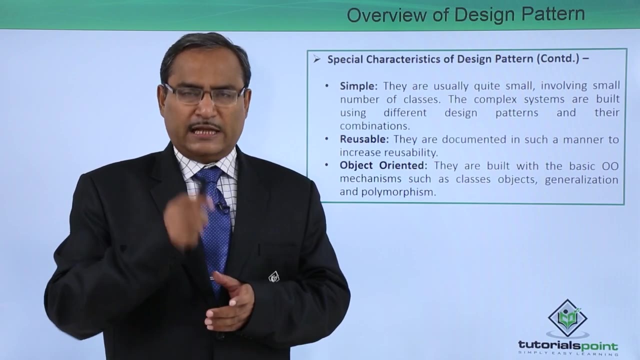 objects, generalization, polymorphism and etcetera. So that is why design pattern has become so popular nowadays for the software developers, so that they can develop softwares in a with a best practices, in a well proven way. Thanks for watching this video.